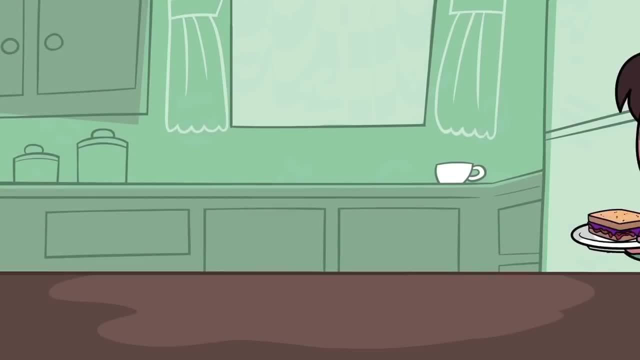 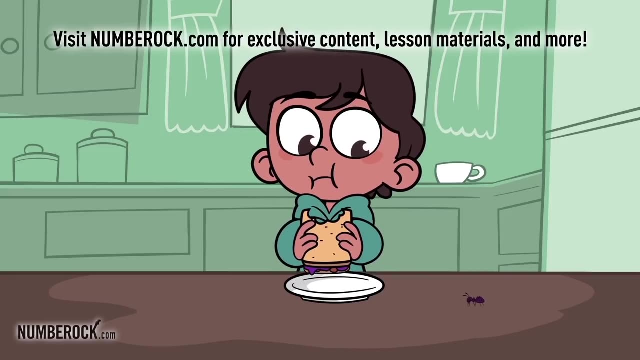 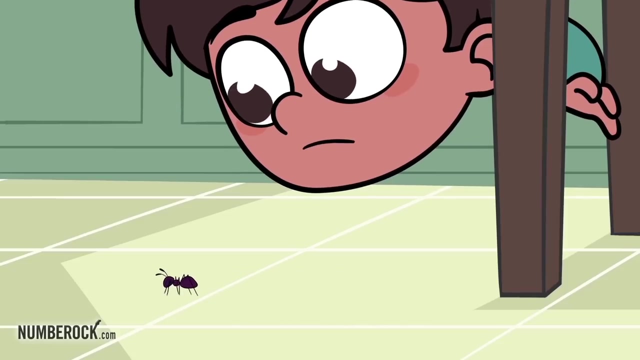 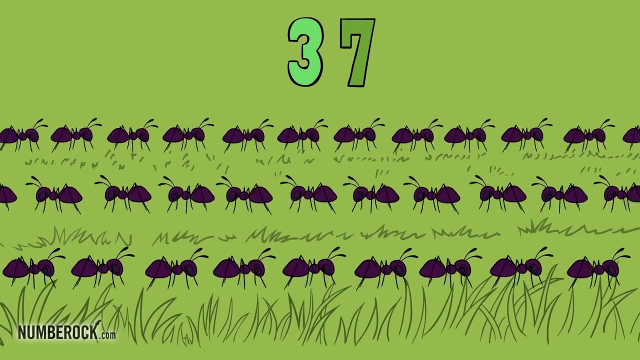 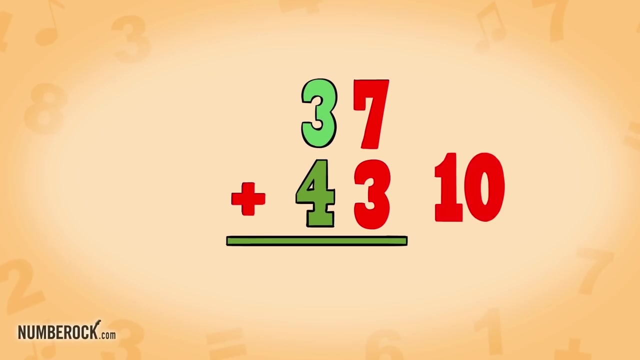 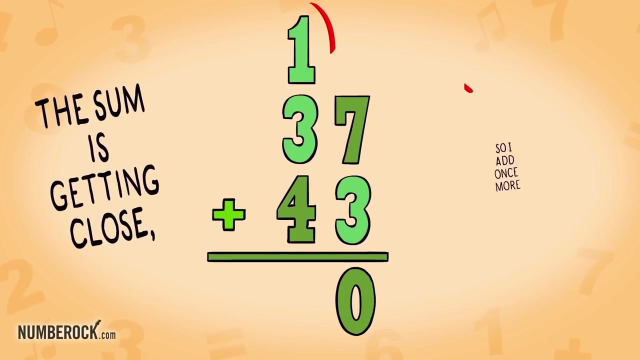 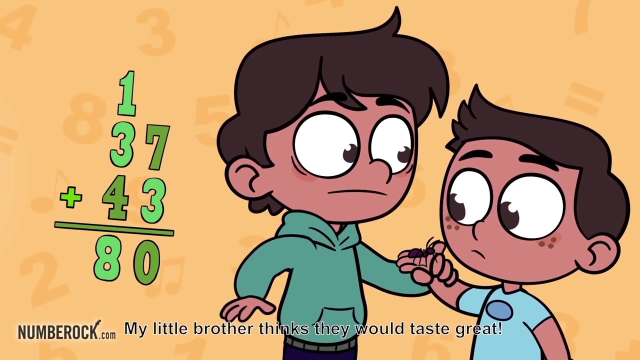 37 ants above ground plus 43 ants underground. 7 plus 3 equals 10. each one of them is my special insect friend. zero stays on the further 10 heads next door. the sum is getting close, so I add once more: 1 plus 3 is 4, plus 4 is 8. my little brother thinks they would taste great. 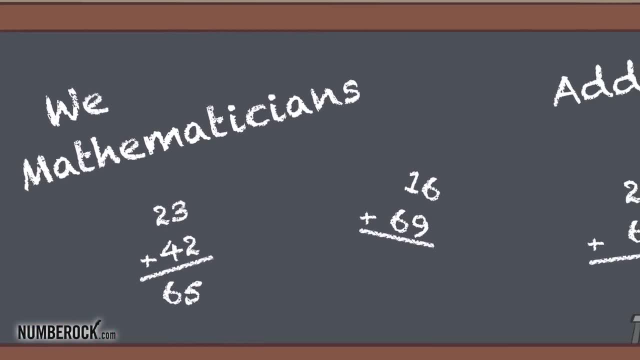 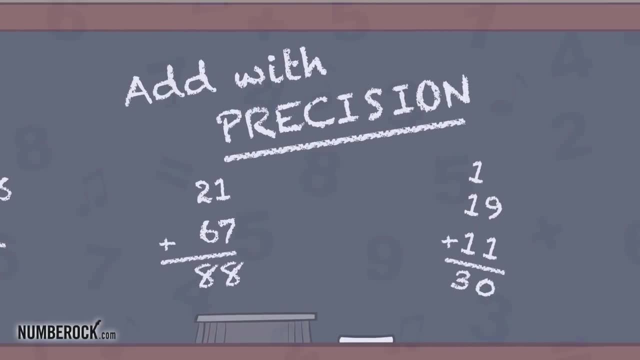 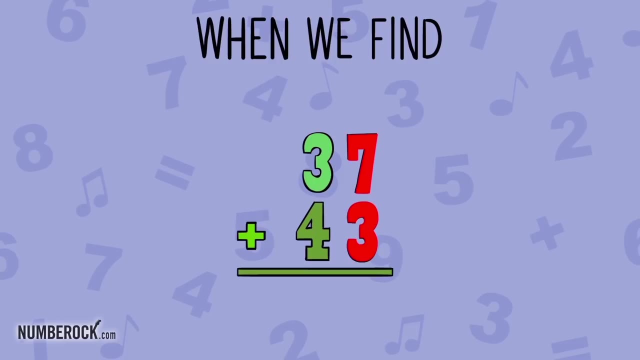 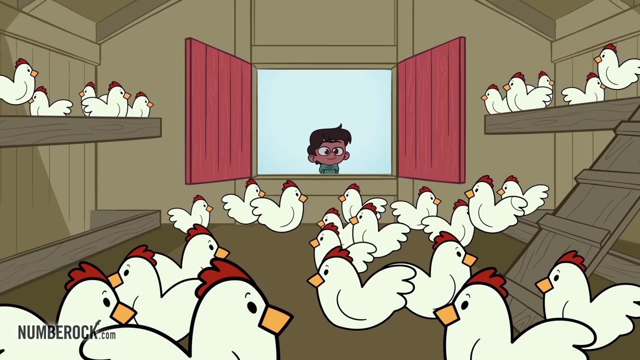 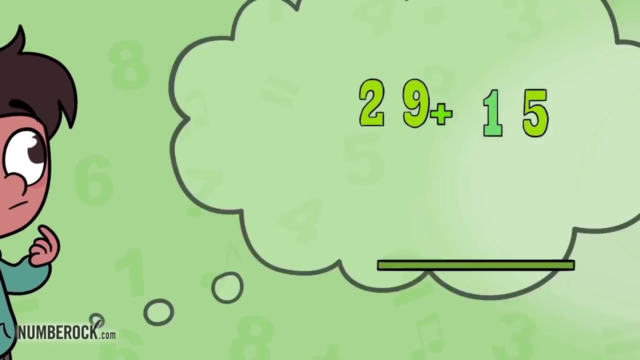 we mathematicians add with precision, regrouping tens when we find double digits. in addition, 29 hens are inside and 15 hens are outside. to find out how many hens are in the coop, we gotta know how to add and regroup. 9 plus 5 equals 14. 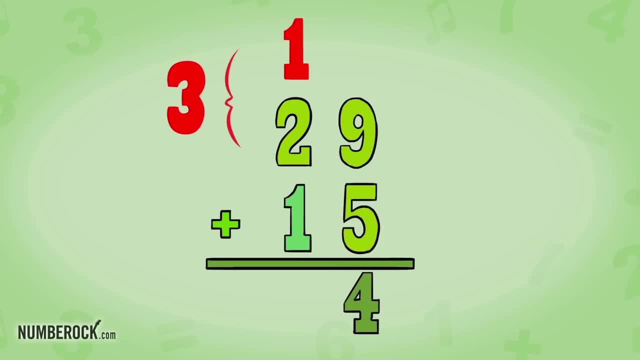 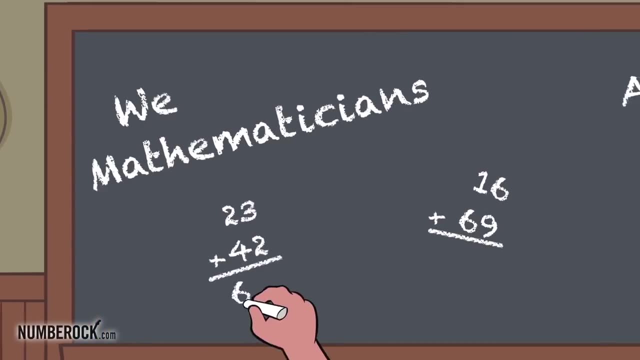 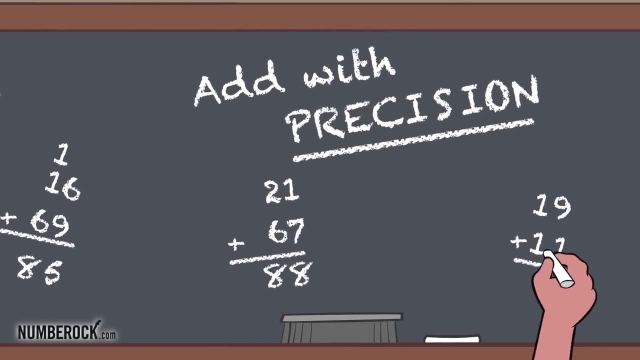 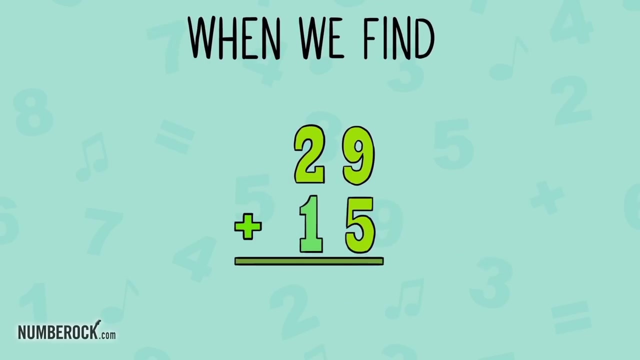 worth of 4. the 10 carries: 1 plus 2 is 3 plus 1 is 4. I wish I had more hands. I wish the farmer was a herbivore. we mathematicians add with precision regrouping tens when we find double digits. in addition, 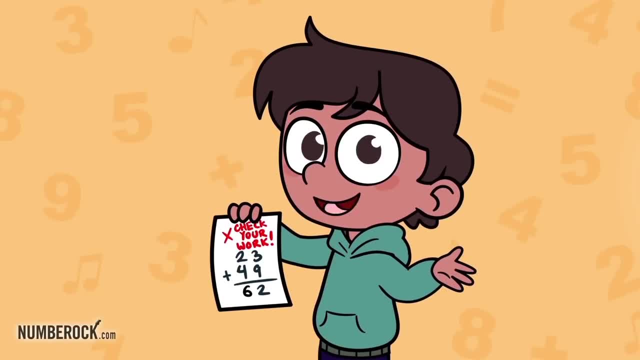 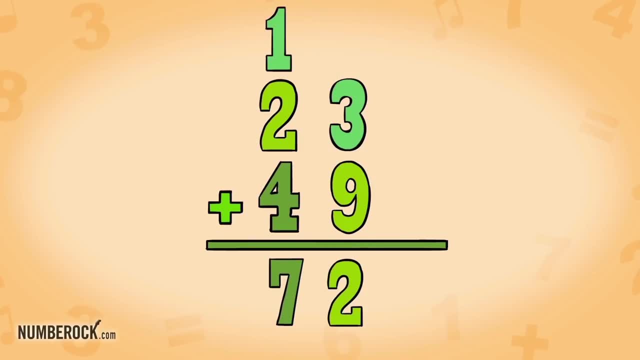 sometimes we make errors. it's inevitable, but check your work and it'll be in due course. the best way to check your addition is by subtraction, the inverse operation. take either addend and subtract from the sum. if you get the other addend, your work is done.